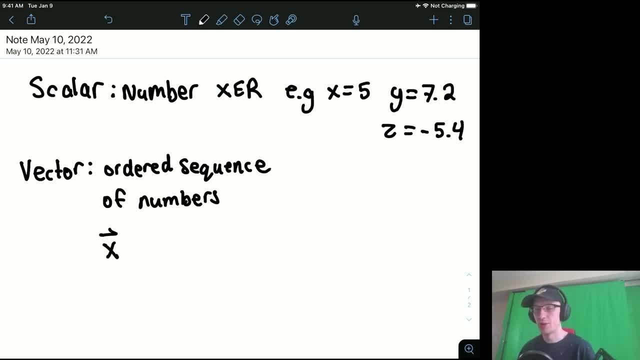 generally we would say something like x with an arrow above its head, so that means it's a vector, and then you'd say it's a member of the real numbers of n dimensions. So basically the n is how many numbers are in the sequence, That's an ordered sequence of two, three, four numbers even. 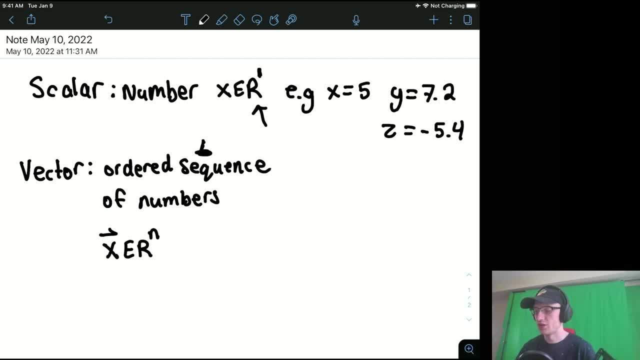 one number, although that's really just a scalar. This you can imagine is kind of. there's an imaginary one up there, but we don't write that. So maybe, for example, you had a vector p, We can use a different letter for that. there's no reason. This is just the general way. we often use x, but 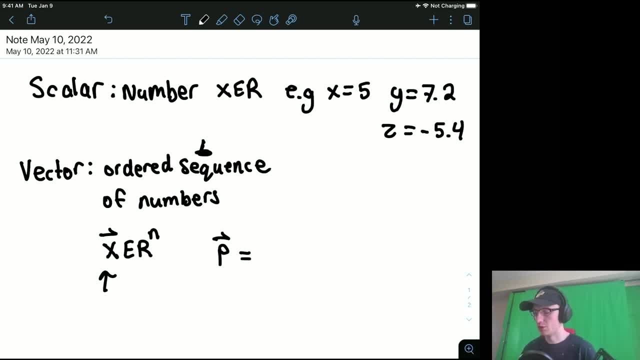 you can also have a vector, p, and maybe that was equal to- and I'll just keep consistent. for example, maybe we had p was equal to- I don't know- 60 and 20.. So maybe this is some sort of a person. and the first component this piece is referring. 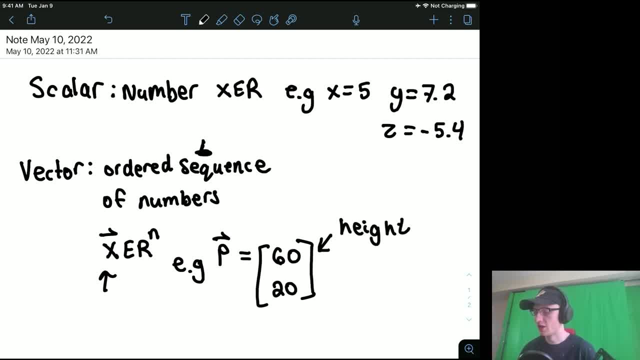 to maybe their height in centimeters. So I'll just say that's their height, and maybe the second piece is referring to their weight. So this is when we would use, say, a two-dimensional vector when we wanted to store information about two different aspects of some object. But you're not limited to. 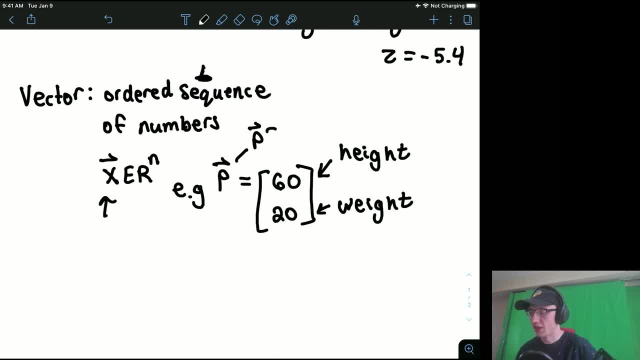 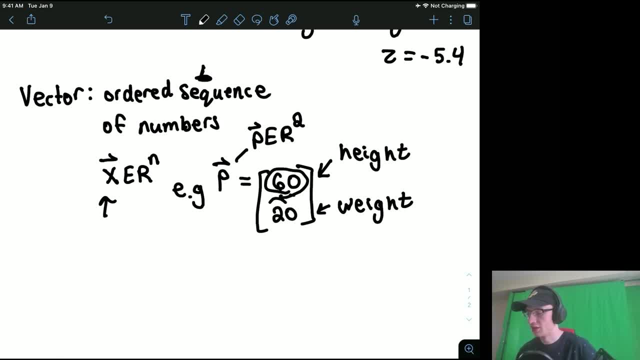 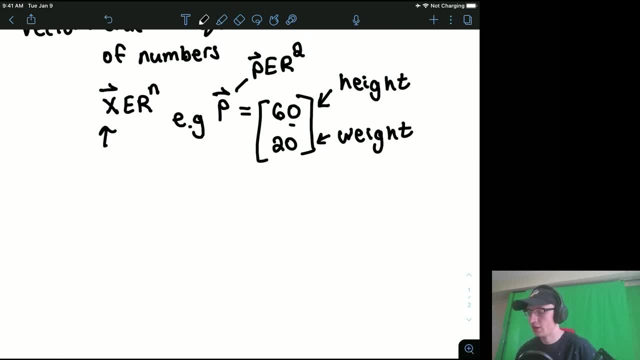 there's two different dimensions there. This is the first dimension, This is the second dimension, But we're not limited to that. We could also have, say, 3 dimensions. So you could have- I'll just call it- z is equal to- I don't know- 30, 20 and 10.. And I'm not going to bother listing what these different. 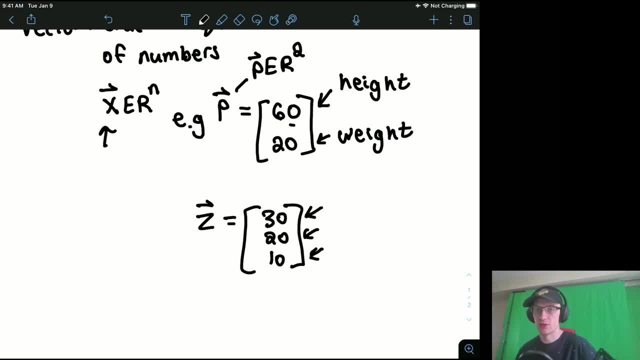 components are. But this would be. you know, if you wanted to store three different things about somebody, then that's how you would do it. And again, technically, Z was a member of the r3 family because there's three dimensions, so you can graph some of these vectors or scalars. 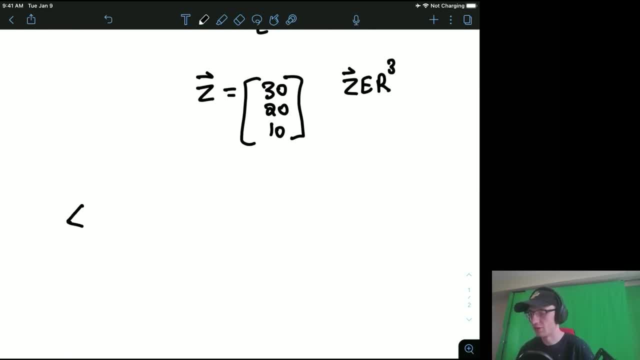 you could always graph a scalar, because it would just be on a number line. for example, if we had this as a number line, maybe this was zero and these were the negative numbers. so this is negative infinity way over here and this is positive infinity over here. maybe we'll just say that. 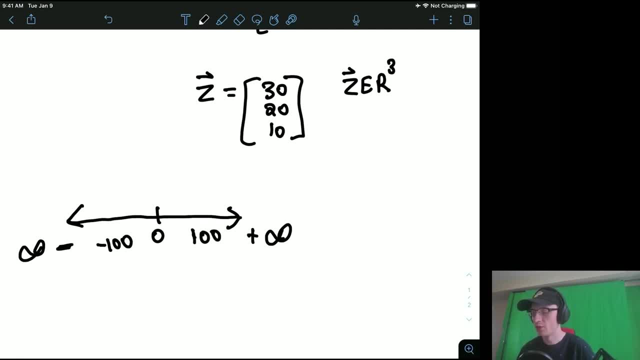 this is a hundred, for example, at negative a hundred. well, if you had some point, maybe it was just the value of three. well then you could plot three right there, although it's really not that interesting. we generally don't plot just scalars or one-dimensional things we generally like. 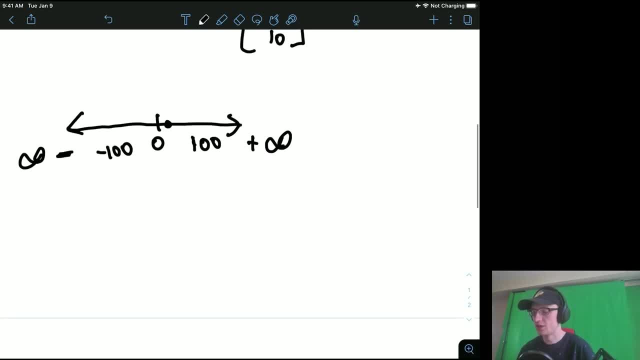 plotting in two dimensions. so if you had, then basically this same thing, but this is one dimension. if you do that two dimensions, you could put one horizontal, and that's generally what we refer to as the x-axis, although in linear algebra you might start to see this is the x1, and then 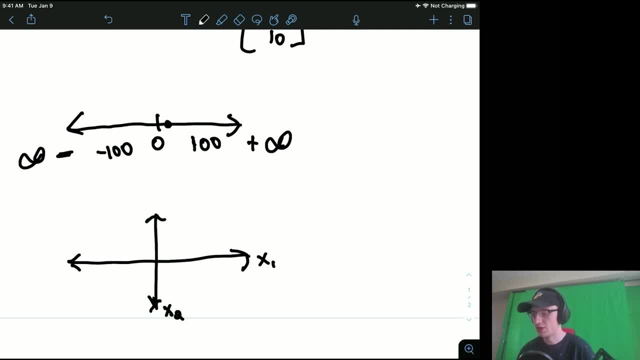 this is the x2 axis. it's really just labeling dimensions. we're used to calling x the horizontal and used to calling y the vertical, but there's really no requirement to do that. but i will actually stick to the the x and y axes because i think it's easier to understand. so maybe if you had a vector which would say: 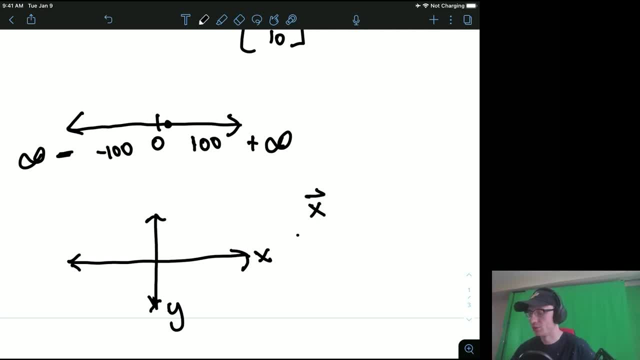 and it's weird, but i'm going to call it x as well. don't get that confused with this x over here. that's just the axis. this is actually the vector. so maybe we had x is a two-dimensional vector, which is three and then four. well, we could plot that as this as well. this is the x-axis and this is the y-axis. x is three. 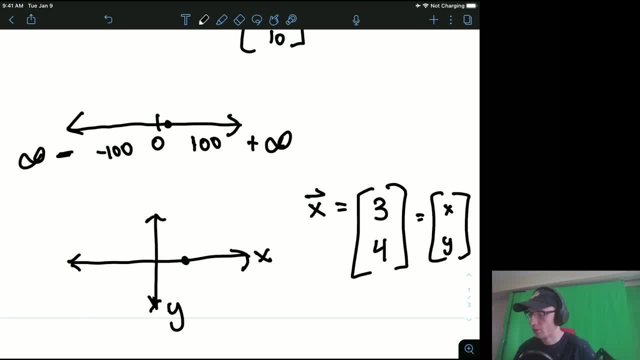 and y is four. so maybe we'd plot that, as maybe three is over here on the x-axis and then four is up here on the y-axis, we would draw the intersection of those things and we'd plot that vector right at that piece there. okay, so now i'm going to move on to specific operations. 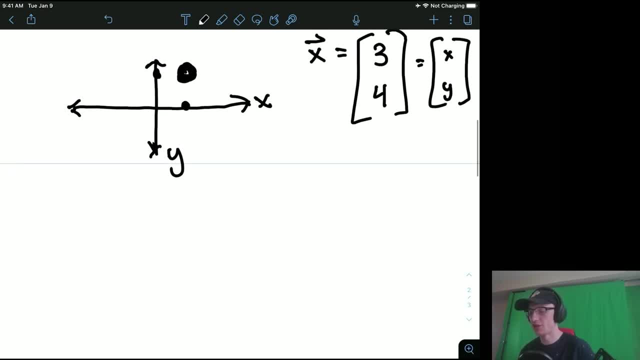 that you can perform on these vectors very, very analogous to you know, we know that five plus five is equal to twelve. no, i'm just kidding, it's equal to ten. and we know that say ten minus four is equal to six. we know that four divided by two is equal to two. we know that there's also 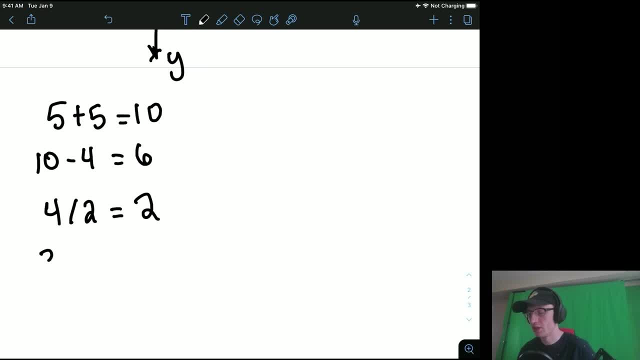 the modulo operator, although we don't use that quite as commonly. we know three modulus. two actually means taking the remainder, which happens to be one. we can do very similar things. i'm actually not going to do this one. we can do very similar things with vectors, and that can be very 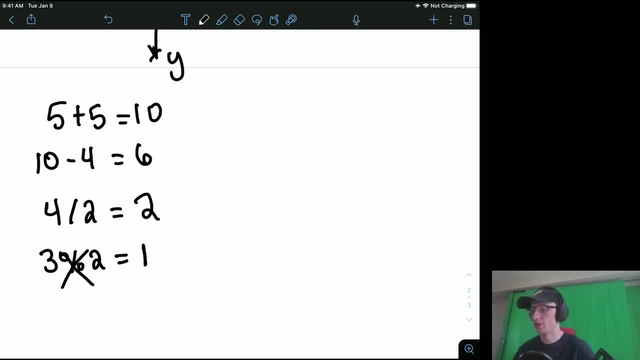 useful. so, for example, you can multiply a scalar by a vector. to show you this, i am going to start writing vectors generally. as x is equal to, we'll write x, 1, x 2 down until x, n, and that is implying that x is actually a member of the rn family. so this is just saying, like we have dot the dot. 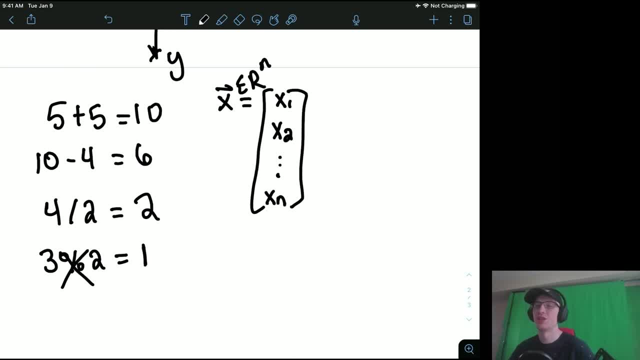 because we don't know how big the dimension is. we're keeping it generic, and so the dimension is n, so n is at least one generally bigger than one. so we're going to start writing vectors, in this case, where some vector in the real boundary, u基本 value, would be x or y. so 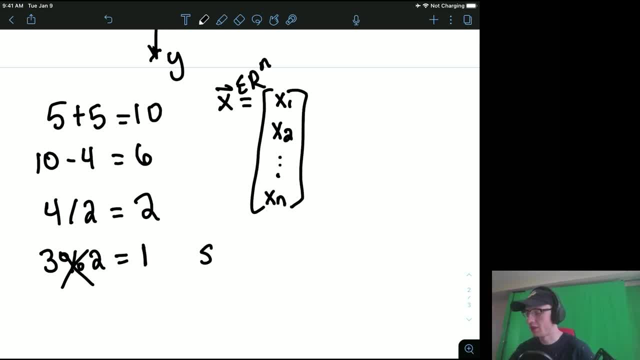 it's going to be x of equal to one or maybe two, and anything below that isNão. you can not like. do some some scales foränn. that would be a measure. we don't know exactly how big these. bigger than one, so at least two. you can think of it probably as at least two. so if we did multiply. 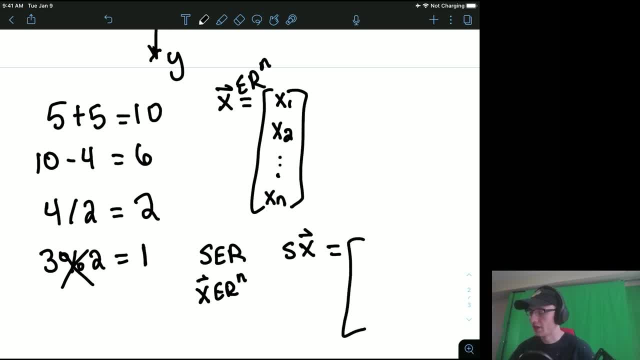 a scalar by vector, that would be s. so some scalar, i'll write it s in the reels. that's just some number and then some vector. we'll write x in rn. so if we combine these things, if we did s times x, well, that is simply equal to well. if x is this thing right here, that is equal to s times x1. s times x2 down until a million. someone is От the sin éo in damage. 1renertx1: 1. you have to take lxx2 as altisto. 1 en amount. x1x2 is none toocmàchäin. 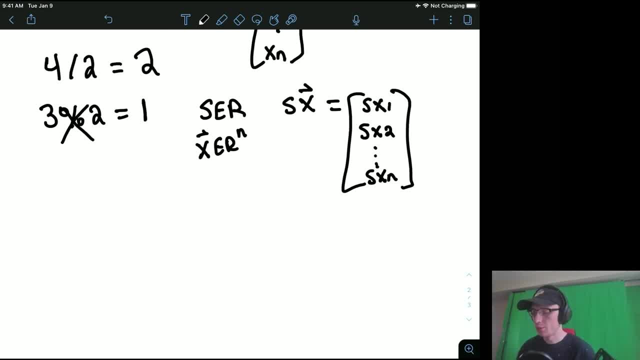 s times x, n. So for example, maybe we did s, x, where s is equal to four and x is the, we'll say it's a two dimensional vector. So that's setting x equal to two. here there's two components in. 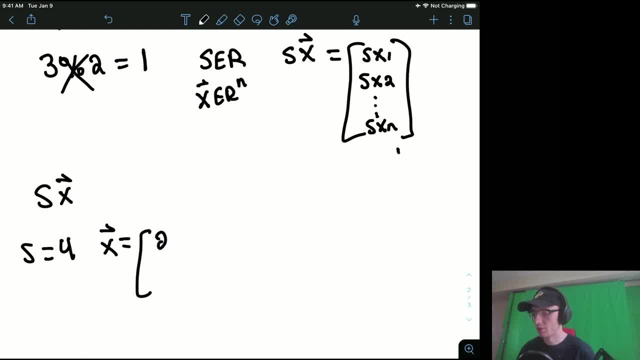 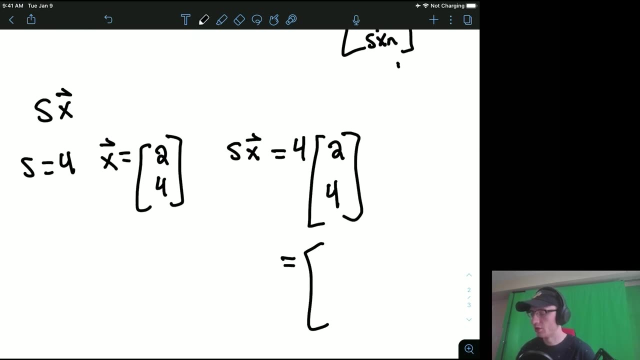 the vector. if we had x equal to maybe two, and then four, well, we could do s x, which is actually equal to replace that with four, replace that with two and four, and then that goes into each component. So that goes four times two. I'll write it like this. we'll see why later: four times two. 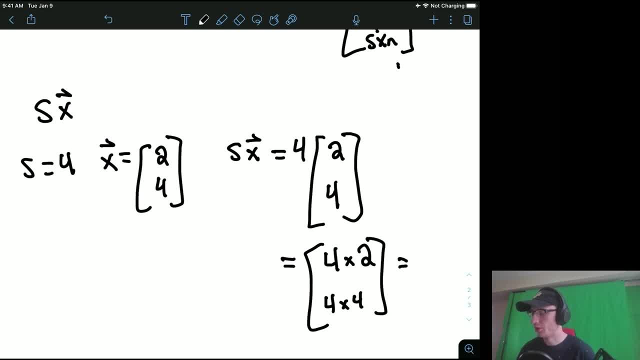 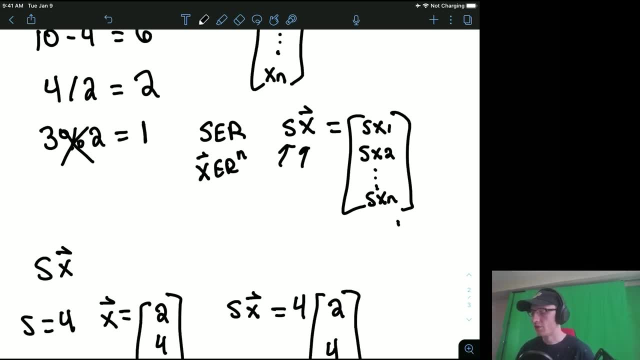 and then four times four, which is just when we know how to do that, it is just eight and then 16.. So all that saying, if you multiply some number times a vector, that means all of those components that we have. we mean these things. it's individual numbers. 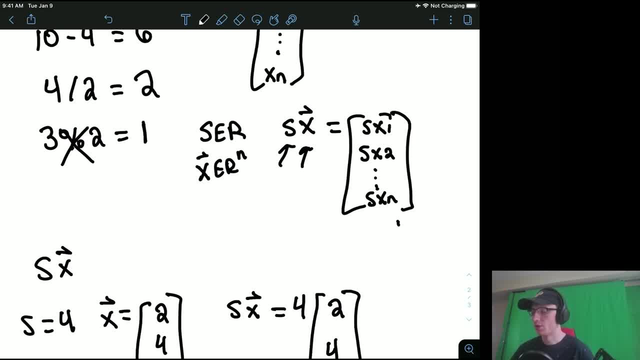 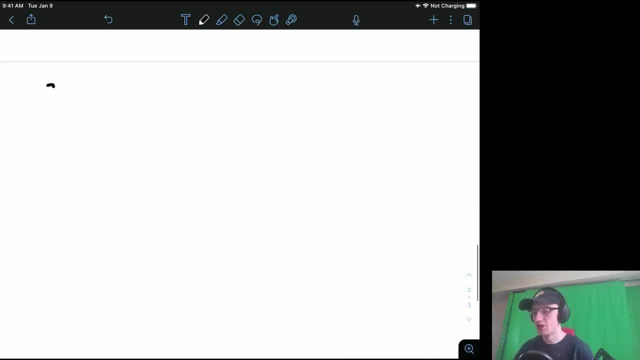 as components. it means that we multiply each of those components by the scalar. Very similarly, we can also add vectors, as long as they're the same dimension. because if you did try to do something like three, two, and then you tried to add that with four, five, six, we would be like 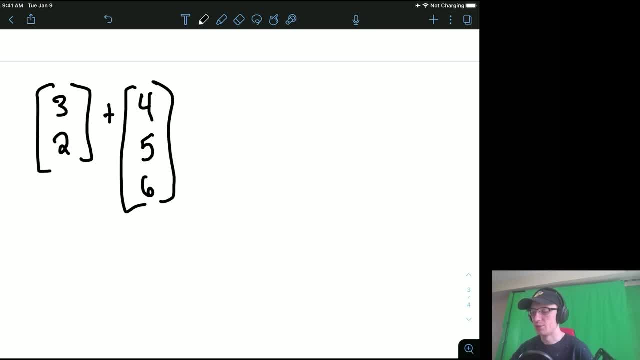 well, what are you talking about? This doesn't line up. I mean, maybe you could have done something like: this is equal to you know, three and four is seven, two and five is also seven, And then I guess six and zero. But technically we're going to be able to do that, So we're going to be able to. 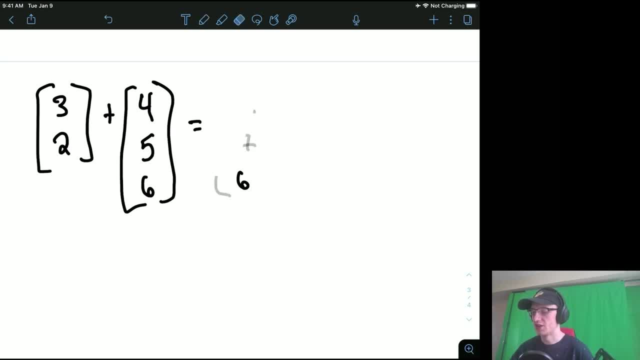 in linear algebra this is undefined, So this doesn't actually exist. we would never do something like this. what you can do is add vectors of the same dimension. So it kind of makes sense. if you had well, three, two and then you were adding all four and five, well, that is equal to the sum. 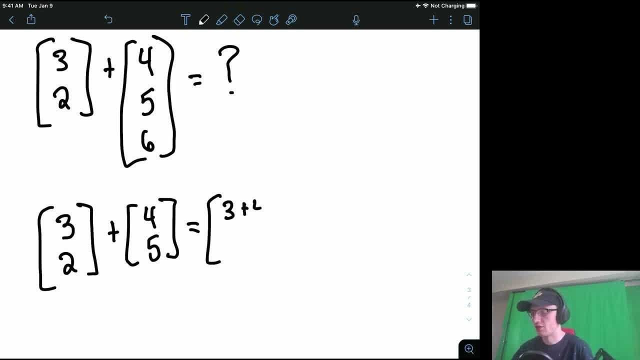 of the components. So that is three plus four, and this is two plus five, which is equal to when we know how to do that. that is seven and then seven. And it's also a two dimensional vector. So if you're adding vectors in a given dimension, 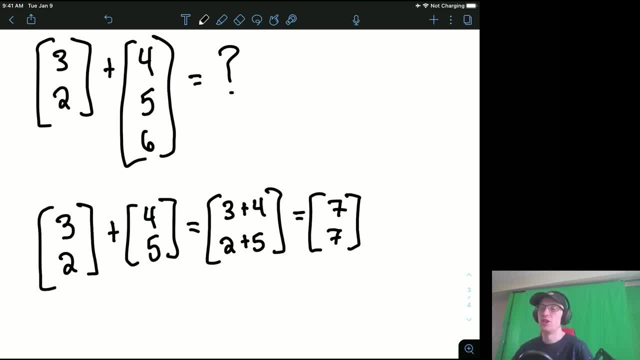 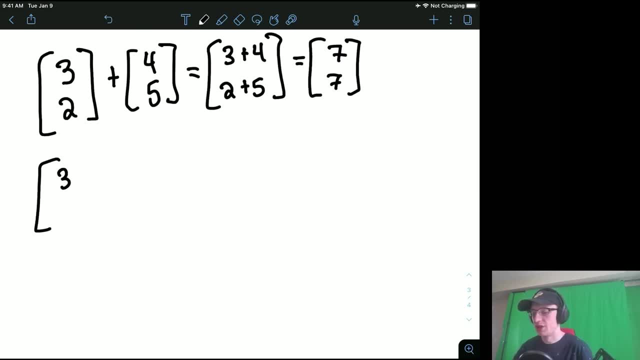 so this one is two. if you're adding vectors in two dimensions, you're going to get two dimensions back similarly, but really is identically the same thing. you could also do subtraction. So if we did three, two and then minus four and then five, well, technically what that is is just 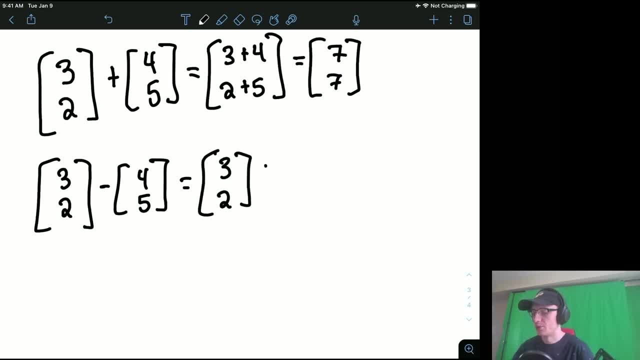 addition, it's three, two. you could place that with plus the negative four and negative five, and we know how to do that. that is three and negative four makes negative one and two and negative five makes negative three. exactly the same thing as addition, but with negative numbers. 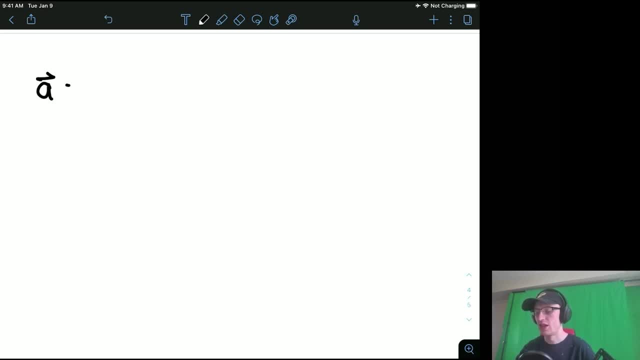 So basically the dot product. if you had two vectors, we'll say: a is equal to four, three. and then we had another vector: b is equal to 10. And then 12. If you did a and then the dot product. 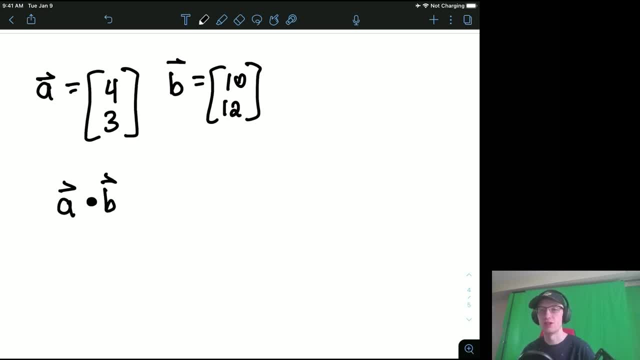 a dot b. that's why I was using that cross, This multiplication, to not be confused with the dot product here: a dot b. So this is equal to: we get the first component of a, which is four. I'm actually now just going to write multiplication. 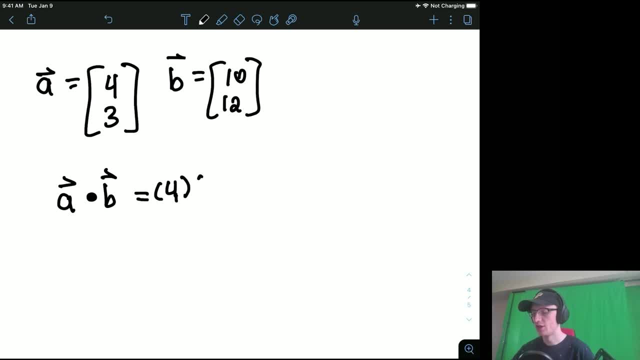 as putting brackets beside each other like this. So four and then 10.. So that's this component times that component. we take those two and then we add that to this component. three times this component over here with b 12.. Okay, 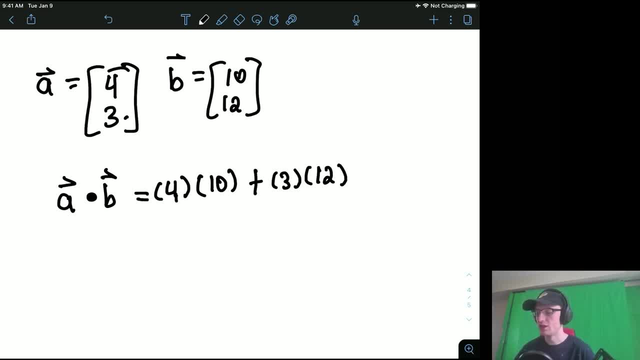 so we take each of the matching components, we have these things here: four and 10, I'm just going to erase the b, even though it actually is b, I'll just put that over there. So we have four and 10 matchup and three and 12 matchup. So four and 10 matchup, three and 12 matchup, and we 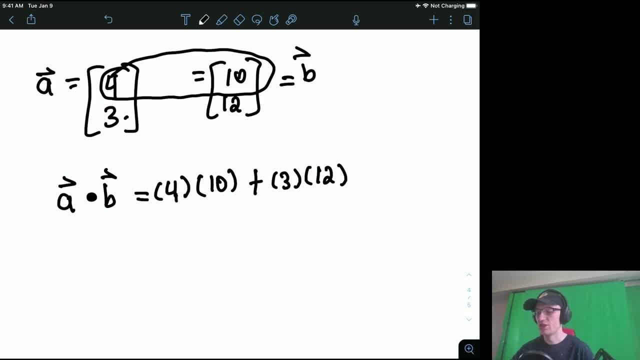 multiply those pieces And then, with the whole vector dot product, we actually end up summing those multiplications, So four times 10, plus three times 12, that is equal to 40, plus 36.. And that is equal to 76.. Okay, so we use the dot product for many reasons And that 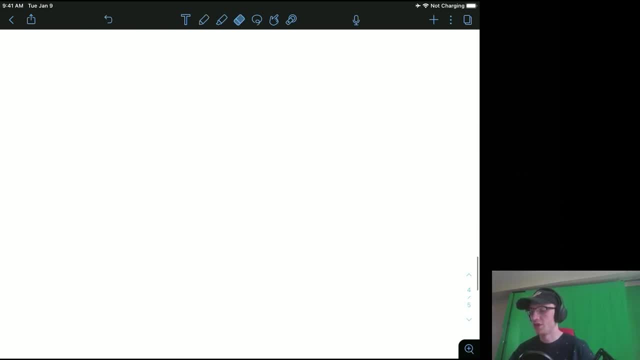 will come up soon. For now I'm going to introduce this new thing, the transpose operation. So if we had x is some vector, maybe it's four and then two. Well, if we had x transpose, so x we write. 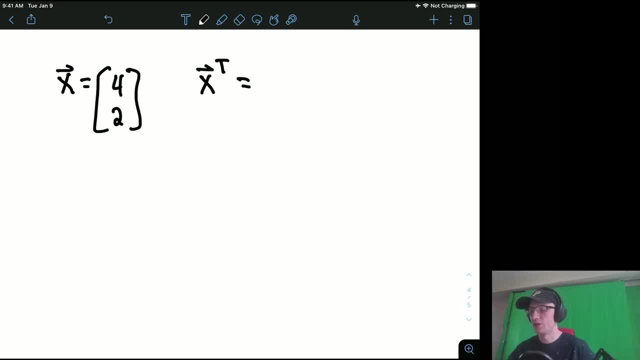 it with a T over here: x transpose. that is equal to actually just a reorganization. it is four and then two like this. Now I'm going to ignore that transpose for now it might not seem very useful. It's like: 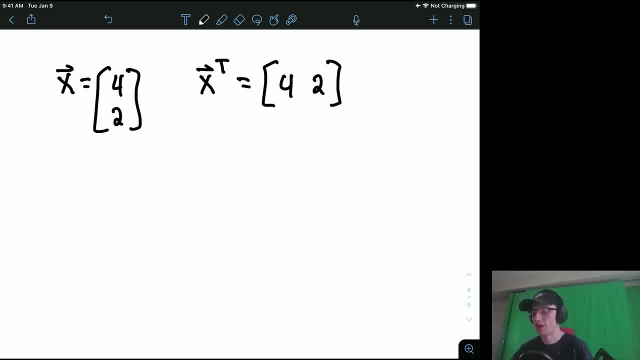 we just shifted horizontally. Well, I'll show you shortly why we might want to do that. So now we'll introduce something called a matrix, or, if you had multiple of them, it would be matrices. we would write it generally similar to the vector, but it's more complicated. x is a member of the real numbers. 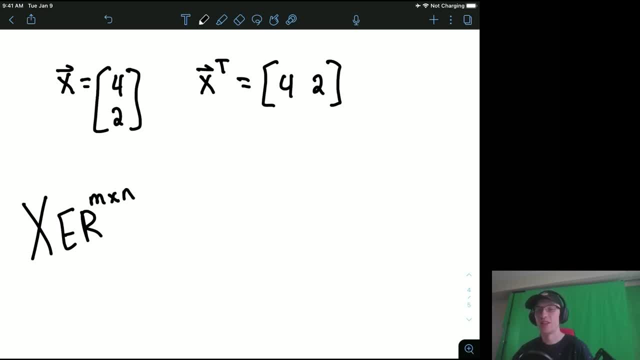 where it's m by n. Okay, we write that up at the top, saying it's basically two axes now. So the x is a vector and our n. Well, that was referring to just going down like this: x one. 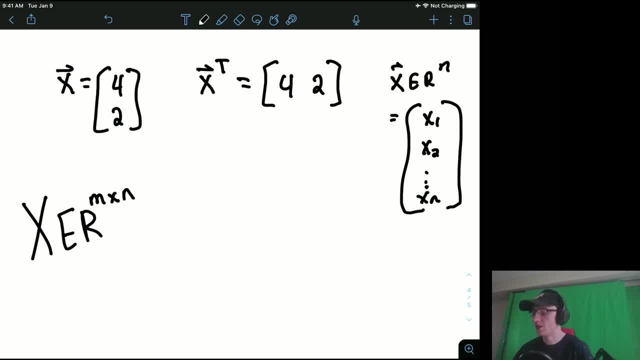 x two until we hit x n. But there's no reason you can't have multiple axes to make what's basically a table of information. So we're going to make that now, And in linear algebra we call it a matrix. So if you were to do this generically, it'd be this big table with the first. 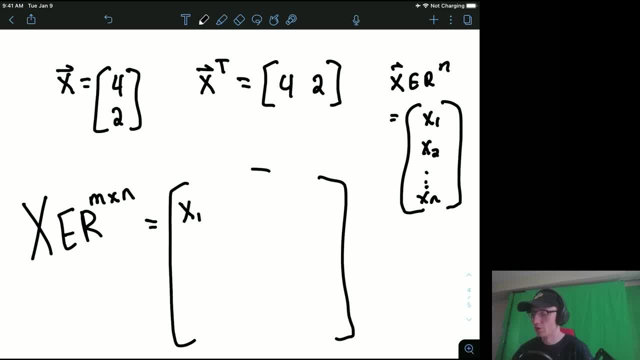 component is x. Well, it's the first row, So row refers to: you know, this is the first row, this is the second row column, so this first column, this is the second column, so the first row, so x1 and then 1, the 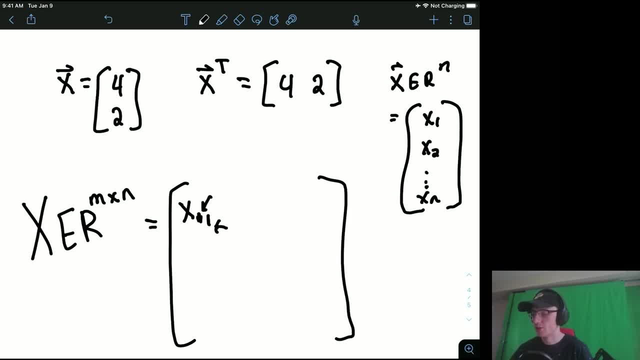 first number refers to the row, the second number refers to the column, so it's x11. if we went down a row, what happens? well, the first number refers to the row, so this increase, this will be x21, because the column stayed the same and it goes all the way down until- well, look what's increasing. 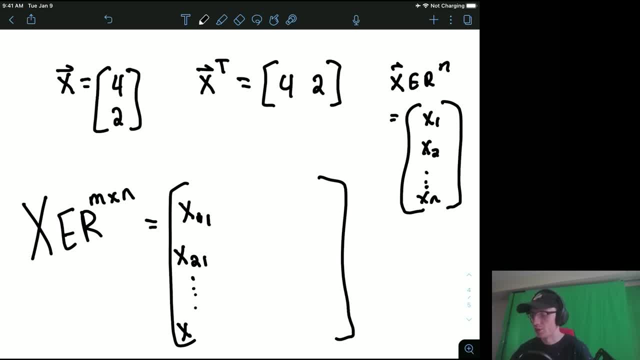 this went from one to two and it goes all the way down. it would help if i wrote m over here and n over here. this will be going down until there's m rows and it's still in the first column. if we moved over one column, it would be x and then, well, the second column, but the row stayed. 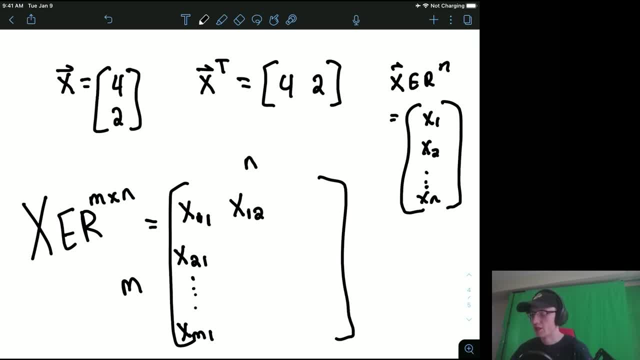 the same. so still the first row, but then the second column and then, if we go down one like that, so the row increased, this will be x2, but the column stayed the same, so x2. that goes all the way down until x. well, it's going to be m still, but in the second column. 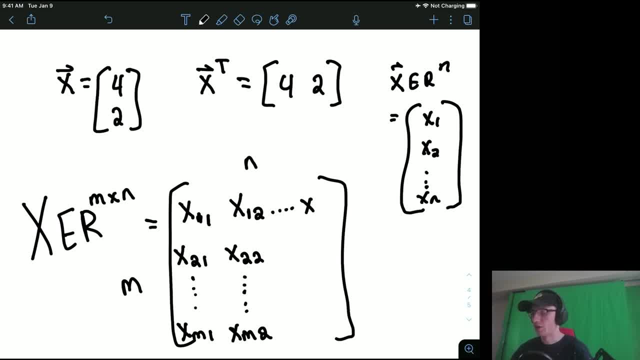 now, if we go all the way across, we actually have: well, all in the first row, so it's still x1. then it goes until x1, n and over here. well, it's the second row, so it's still x2, but now it's x2. 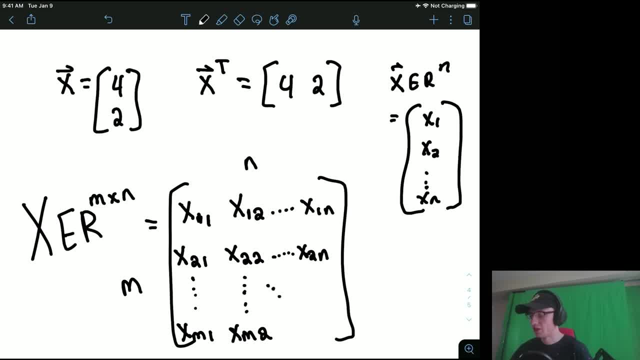 n, the last column. then we generally write it like this: just dots, all leading up until the last component, where that has to be the final row, the final column, and then we go all the way down until the column. there is m rows and there is n columns, so it's x, m, n in the corner. so just an example. 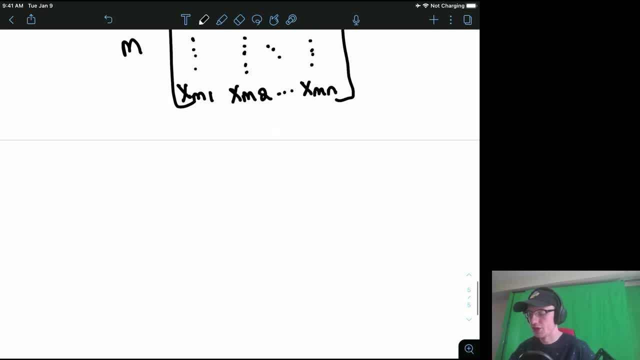 maybe we had some matrix, which is really just a table of information. maybe we had x as a member of the three by two family. that means it has three rows and two columns. we had that, maybe equal to maybe one, two, three, and then there's two columns, so it'd just be maybe four, five, six. this is. 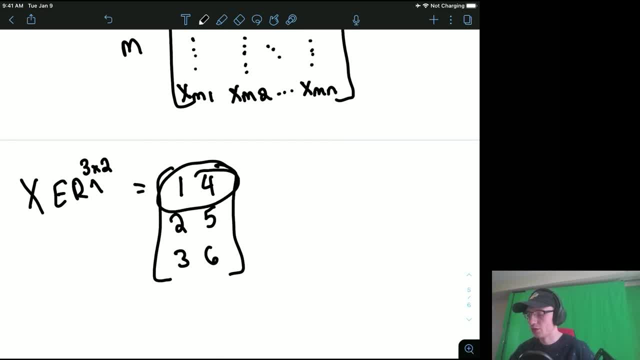 perfectly valid. there's three rows and there's n columns, so it's still x1, n and over here. so we have two rows, three rows, one, two, three and there is two columns. so one, two columns like that. now you definitely might be wondering why suddenly we made n, like n was going vertically here for 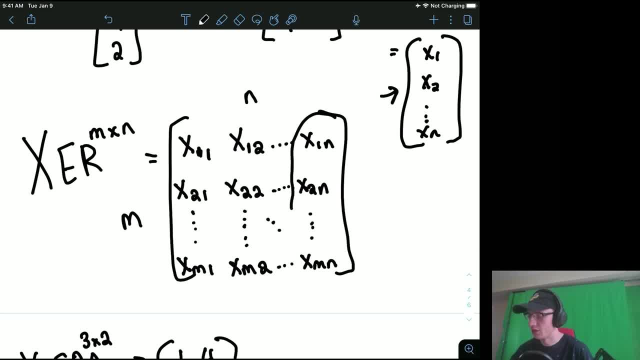 when it was a vector and so that would kind of make sense for it to go until this is n rows. except i actually did m rows and then n got stuck in the sideways in the horizontal format here. i'll show you that very shortly, but for now i'll show you that. 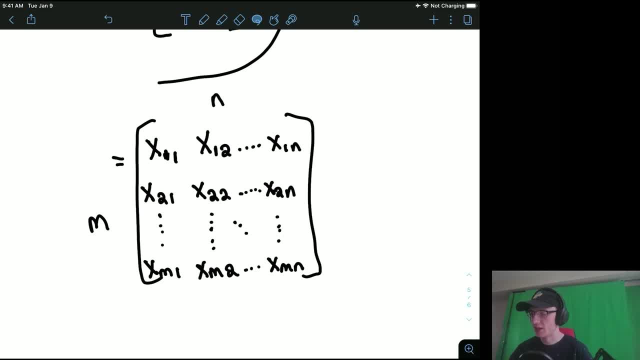 we can actually write a matrix. okay, sorry, i just copy pasted that x over here, so this is actually the same x. x is in the reals of m by n, so we could actually rewrite this if we wanted to, as if we treated each row, for example, as a vector. you might as well. a vector is a sequence of. 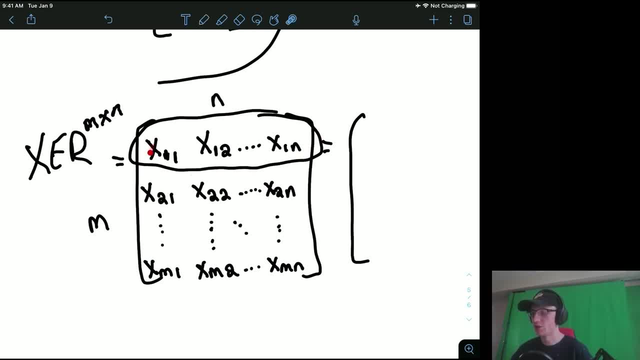 numbers. so the row is all staying the same, and so it's just a sequence of numbers in a row, but it has n pieces: one, two up until n. well, we can take advantage of that, and we can actually write a matrix like that, and so we could simply write this as well: this would be x1, because you know this one. 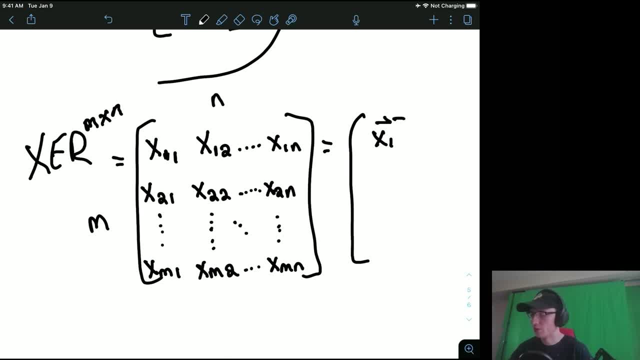 is staying the same x1 and then transpose. so if we made that a vector where it just has n components, that's x1- transpose, and same thing over here for these pieces over here, well, we could easily write that as x2 transpose, and so this goes all the way down until, well, it's the mth row or the last row. 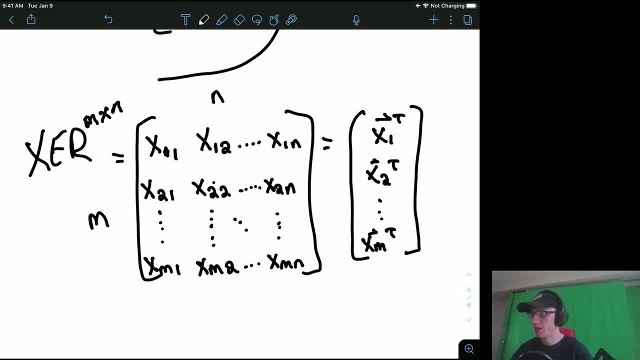 it's transpose, because that's how it was writing horizontally, like that, if we didn't have the transpose, that would then kind of picture them all crumbling down like this. that wouldn't make much sense. it goes horizontal and so it kind of fills out like that. so now i can define matrix. 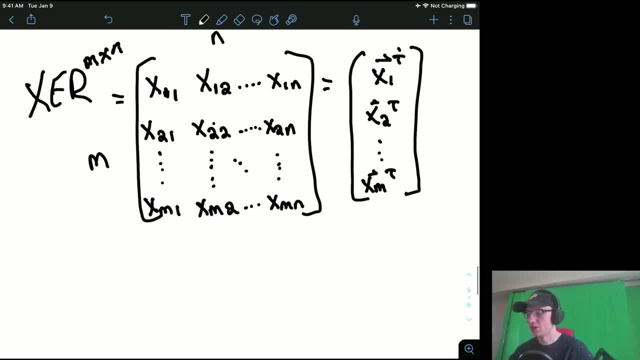 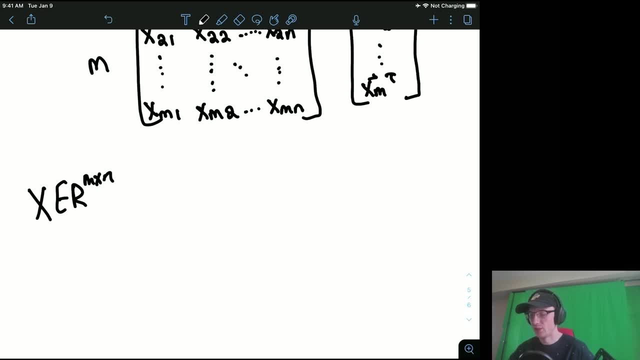 vector multiplication: the multiplication between a matrix and a vector. if we had maybe one matrix, we'll call it: x is an r? m by n, and if we had a vector, i'll use a different letter. a is in the reals of n, and if we had a vector, i'll use a different letter. a is in the reals of n, and if we 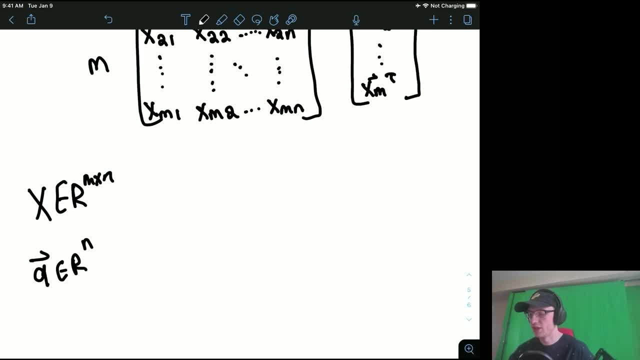 had a vector, i'll use a different letter. a is in the reals of n, and if we had a vector, i'll use a. it has to be of dimension n and i'll show you why shortly. sorry for the crazy jump where i just changed headphones. sorry about that. we can do something called matrix vector multiplication. 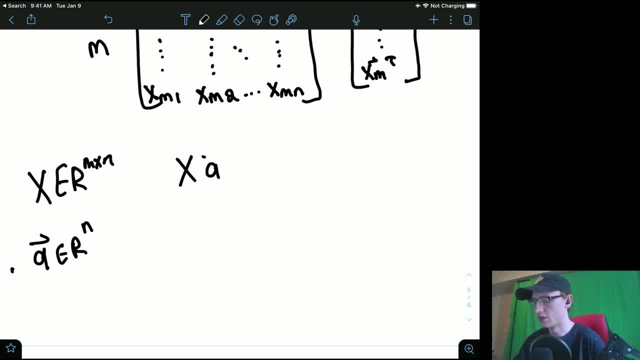 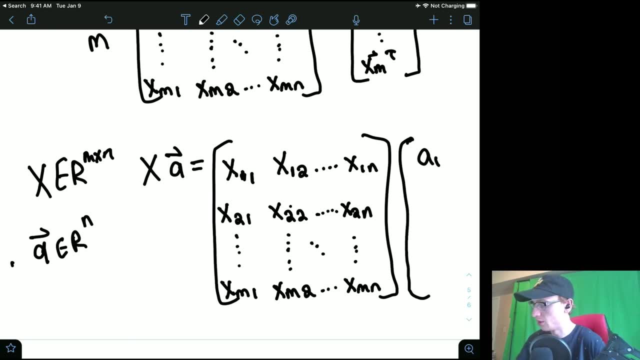 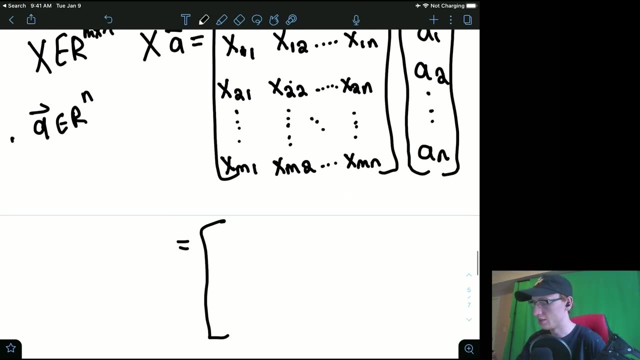 where we have a matrix on the left and a vector on the right. so that that looks again, i'll just copy this off screen. that is x, the matrix, and then you write the vector a, a1, a2 up until a n over here utilizing the transpose and the dot product. this is just x1- transpose, as we. 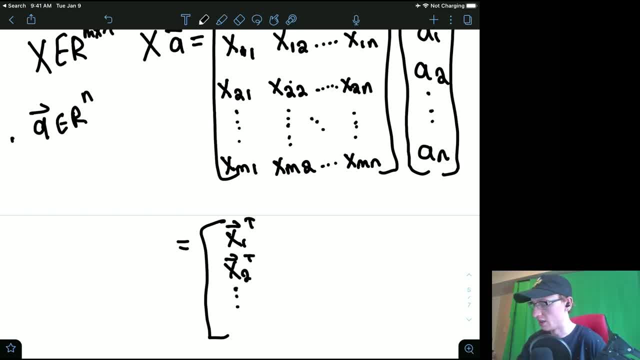 x1 transpose and the dot product. this is just x1 transpose, as we saw, x2 transpose and then xm transpose. we've already seen that, so that's nothing new. and then i'm just going to write that vector again: a1, a2 up until a n, and i'll show you in. 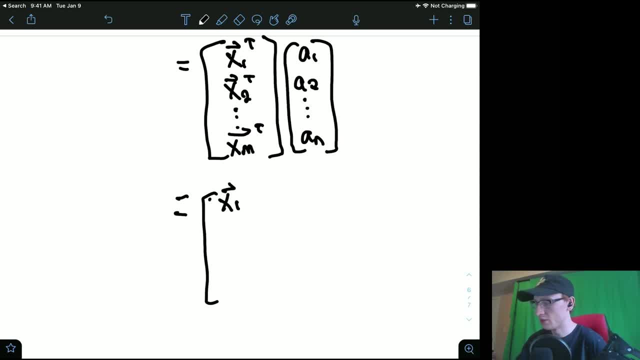 a second. we actually don't even need to have a written out like this. we can just have x1 transpose, x2 transpose, up until xm transpose again. nothing changed there at all. and then i'm just going to put a back here like it was at the beginning, because what this is all about is that we have 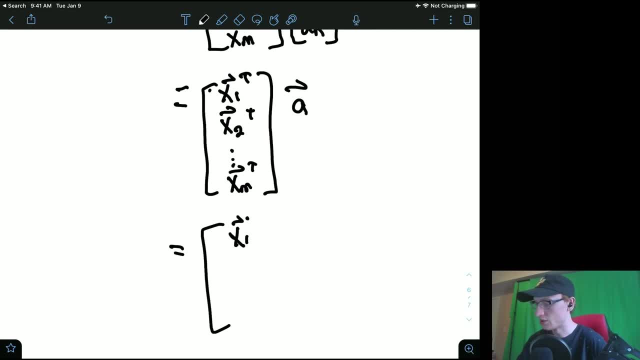 all actually equal to is simply x1 transpose dot a, and then x2 transpose dot a, and then all the way until xm transpose dot a. we just take that vector a and we do the dot product with every single row, and so that's going to leave a vector with m dimensions. because each of these things, this is 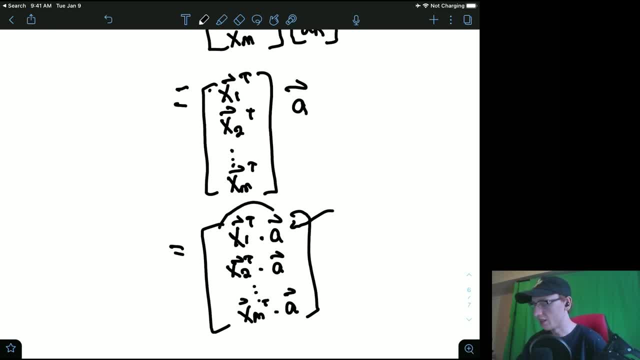 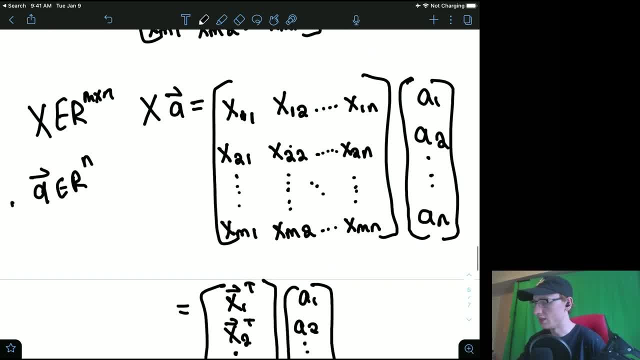 an m dimensional vector and all of this, this very complicated thing that just bottles down to taking this vector here. so, whatever we have over here, we take that vector and then we dot product with this row here, and then after that we take that vector and we dot product with that row there. 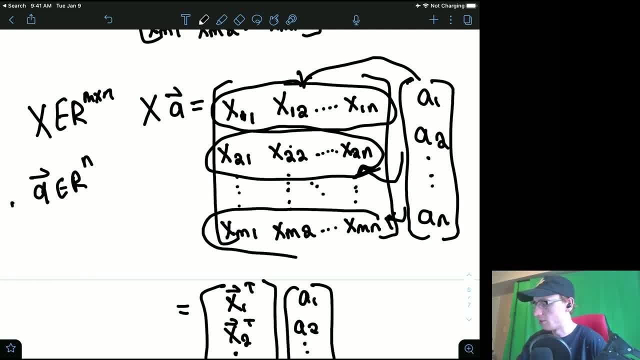 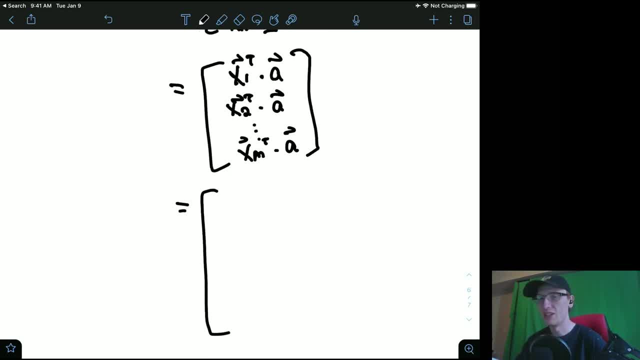 and we do that every single time. the exact same vector. we dot product that with every single row to produce an m dimensional vector. that's it what it technically is, without any sort of math hiding it with any symbols. so if we turn the dot product into what it actually means, it's x11 times a1 plus x1. so i'm keeping that same. 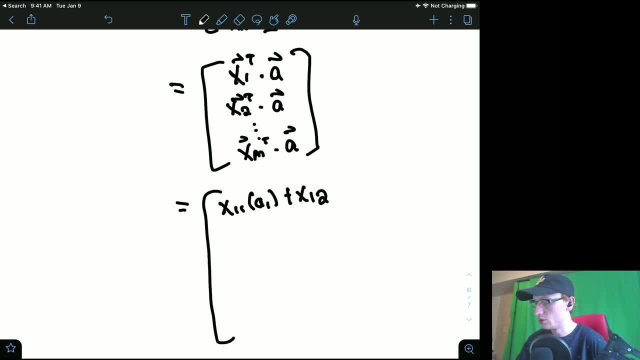 number, because this is for each row, so x12 times a2 plus dot dot dot. until how many columns do we have? well, it's going to be still first row, but then n columns, so x1, n columns, so x1, n columns n, and then i'm just going to do, without the brackets, a n, like that, and then the second row. 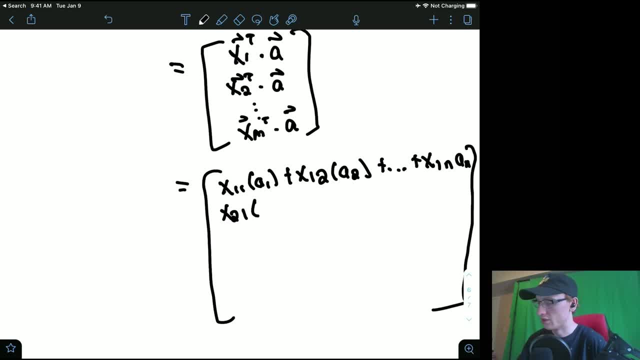 x21 times a1, it's the same a1. plus x22 times a2, it's still a2, and then plus all the way until x, it's still the second row. and then there's n columns, then again a n. like that we do that. 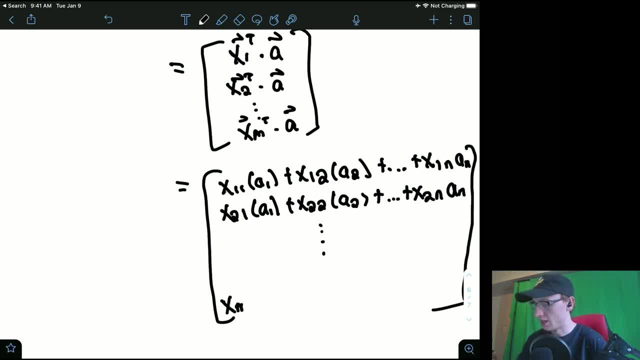 all the way down until we have m rows. so x m1 times a1 plus x m2 times a2, plus dot dot dot, plus x m n times a n, and again there should be brackets around this a n, it just means multiplication with that particular unit, so i'll try to put. 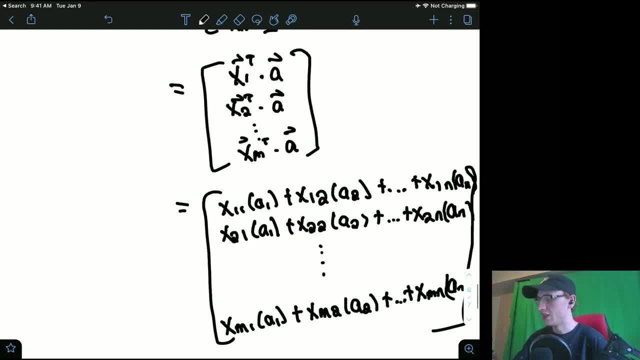 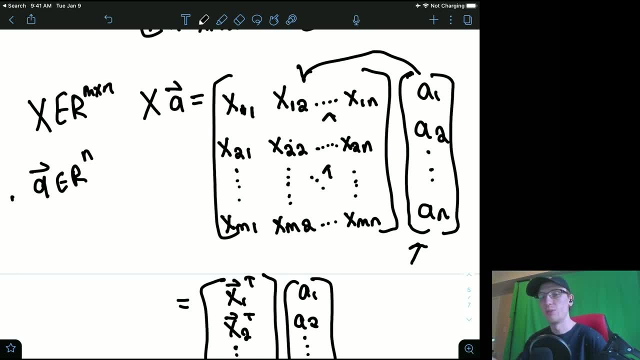 that in there. basically again, no matter how you want to say it, you take the vector on the right, you take the vector on the right and then you dot, product it with each individual row. and we do this in many different applications in machine learning. so say, for example, we had some matrix. 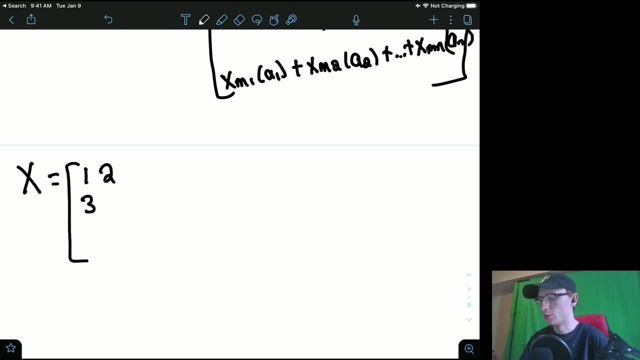 and we set that equal to maybe one, two, three, four, five and six, and then we had some vector a. so a is equal to what has to have two dimensions. we have to be able to dot, product it with that horizontal, so it has to be something like maybe three and then ten. so if we did the matrix vector 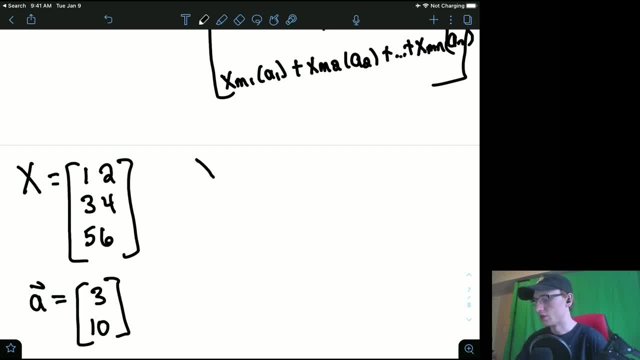 multiplication, which is the effect, which is the matrix on the left and the vector on the right, which is replaced with what they actually are: one, two, three, four, five, six, and then the vector, which is three and then ten. we would do the dot product and so this three.